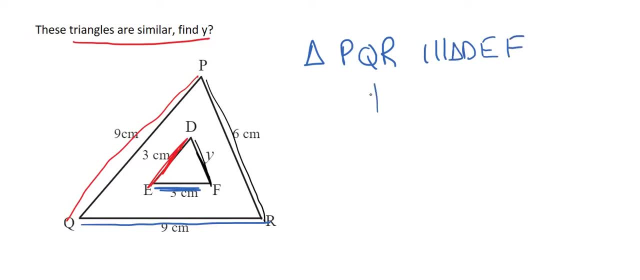 letter would be F. It's very important that you do get this order correct. So the first triangle, I just chose PQR, and then you must make sure that these letters go in the correct order, Because what did we learn in the previous lesson? We learned that 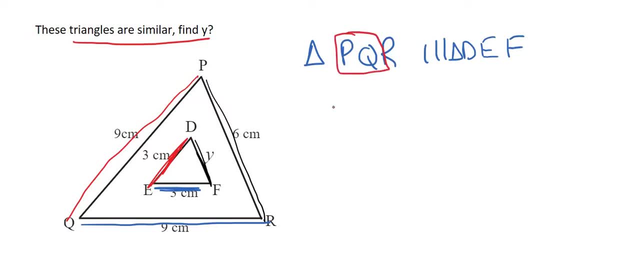 if two triangles are similar, then it means that this one, PQ over this one, would always equal a certain number, and that number would have to be the same as, for example, this one PQ over this one And that number, whatever it is, would have to be the same as these two over these two. So PR over DF. 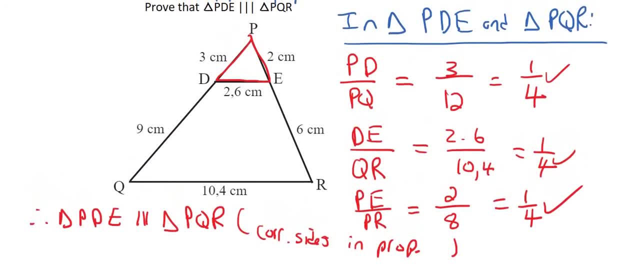 Okay, we know that those must be the same. Here's just a flashback to one of our last lessons. We know that when you divide them, you get a quarter. then when you divide these two, you get a quarter, and when you divide these two, you get a quarter. So 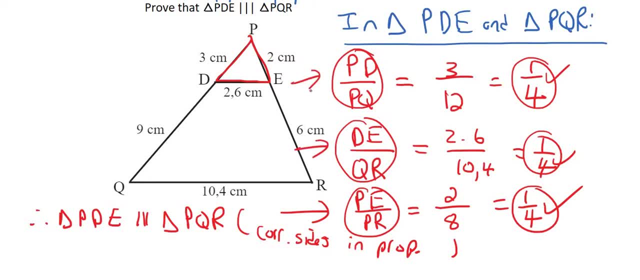 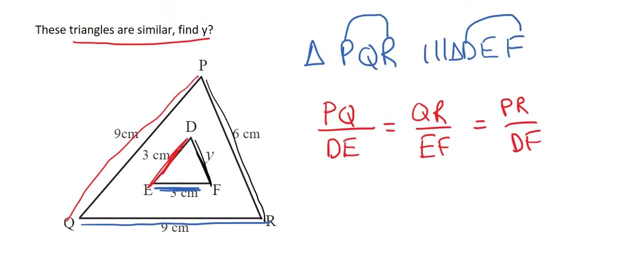 what it means is that these three things are all the same, and so that's what I've just written out of here. I've said that they are all the same. That's the difficult part. Now. all that we need to do is fill everything in. So PQ is nine DE. 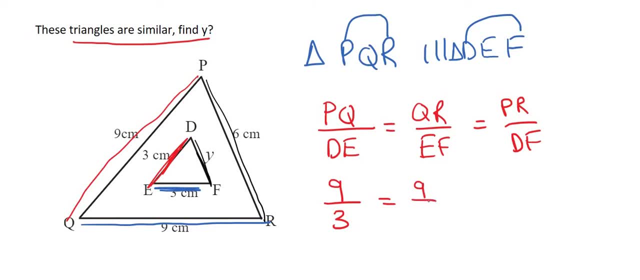 is three, QR is nine, EF is three and PR is six, and DF, we don't know. So now what you you do is you just try find y, So you only need to choose two things at a time, So we could for. 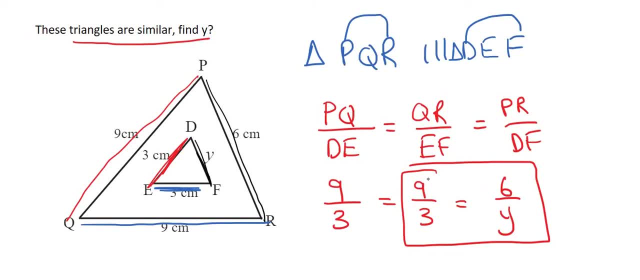 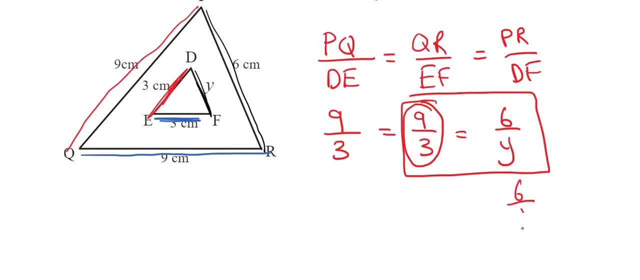 example, choose these two over here. So if you just look at this ratio over here, you can see that nine divided by three is three. So we could say six over y should equal three over one. Now we can see that to go this way you'd have to multiply by two. So to go this way you'd also multiply by. 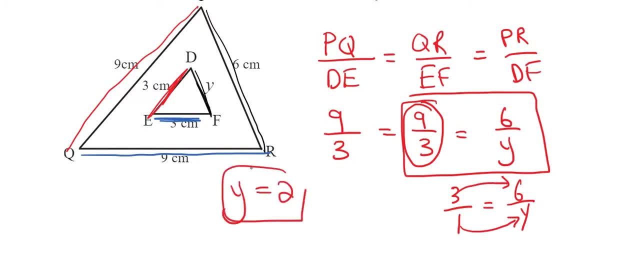 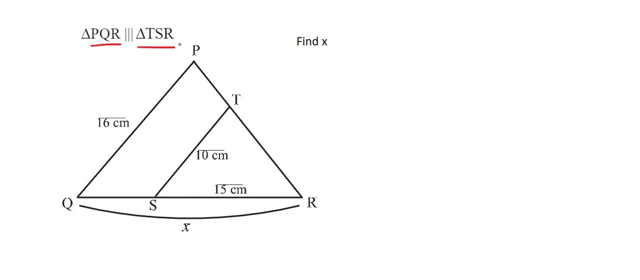 two, And so this means that y has a value of two. Moving on to the next one, Here they've given us the two triangles and they've told us that the two triangles are similar. So what I would do straight away is I would form my three ratios. So that would be pq over ts. That should always be. 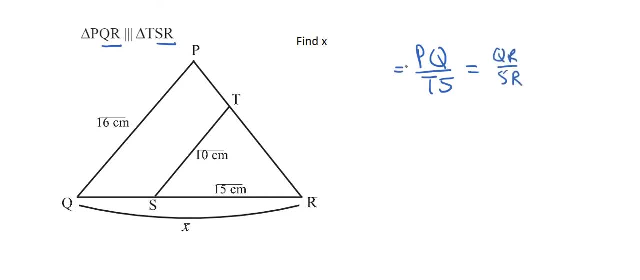 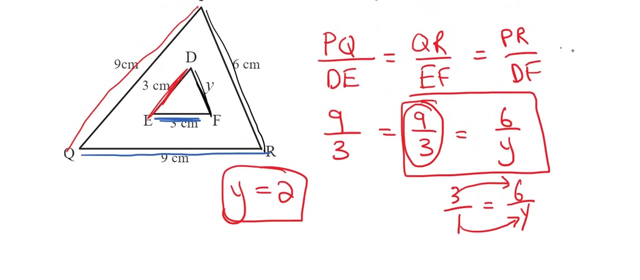 equal to qr over sr, And I'm just going to add the other one in the front just to save a bit of space. That would be pr over tr. So pr over tr over tr. Now your reason for this. I should have actually given a reason up here when I wrote these. 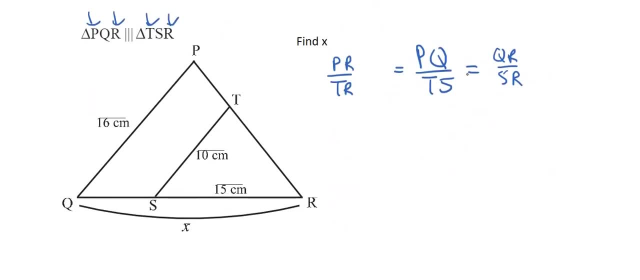 out. There is a reason for that. It's because the triangles are similar, but specifically, you would say that the corresponding sides are in proportion. Why can we say that? Because these two triangles are already similar. Now, what you do is you just go full information in, So pr. we don't know what. 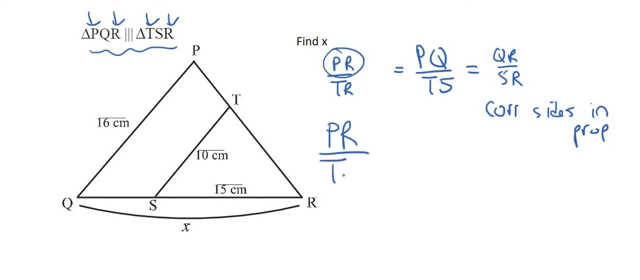 that is, so we just leave it. tr. we don't know what that is, so we just leave it out. pq is 16.. ts is 10.. qr is x And sr is 15.. There we go, So now we don't have to even use this one, So we. 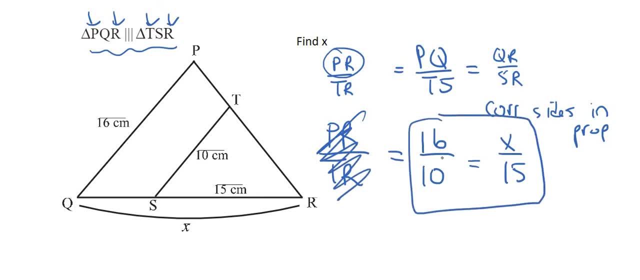 just use these two over here, And so 16 over 10.. If you type that in on the calculator, it will be 8 over 5. And so now we can see that the ratio to go from there to there you would times by 3.. 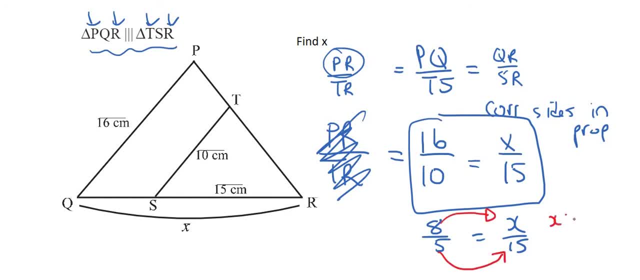 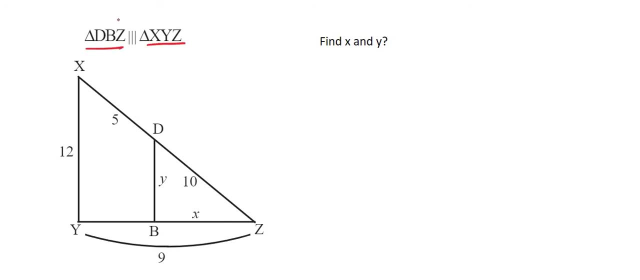 And so to go from there to there, you also times by 3. And so x would be 24.. And then here's the last one. So they've told you that the two triangles are similar. So you write out the ratios first, And so you say db over xy would be the same as 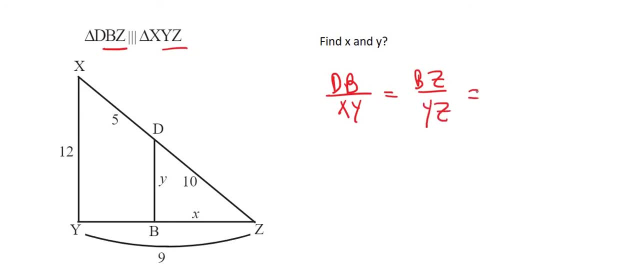 bz over yz, And that would have to be the same as dz over xz. Now you must give a reason. That's because the corresponding sides are in proportion. Now you just go full everything in. So db is a y, xy is 12. bz is x And yz is 9.. dz is 10. And xz is 9.. 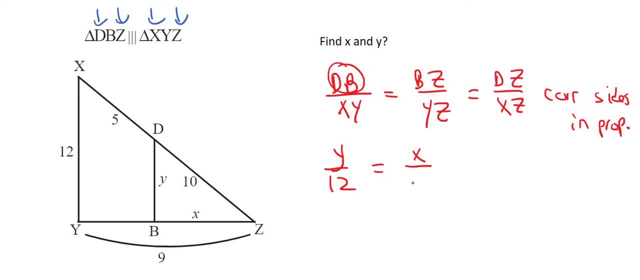 So we just go full everything in. So db is a y, xy is 12. bz is x And yz is 9.. dz is 10. And xz is 9. is 15.. Now to find x, for example. you wouldn't choose these two, because there's an x and a y.